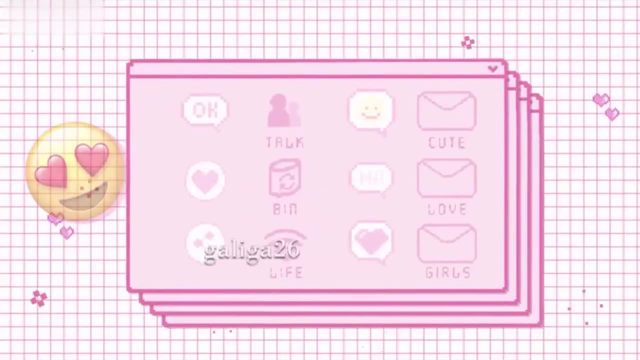 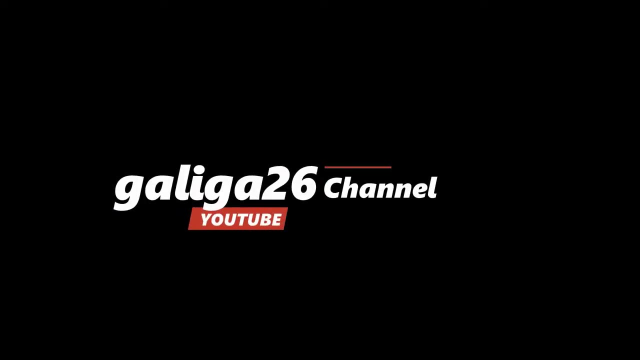 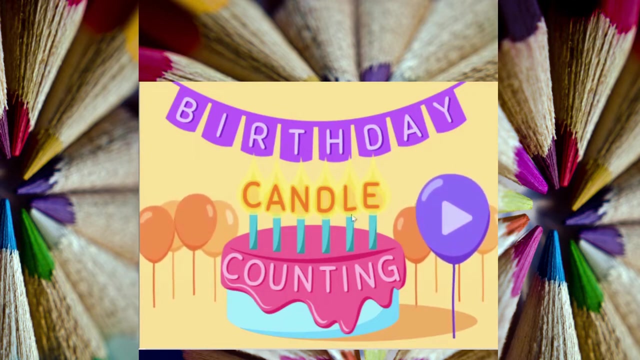 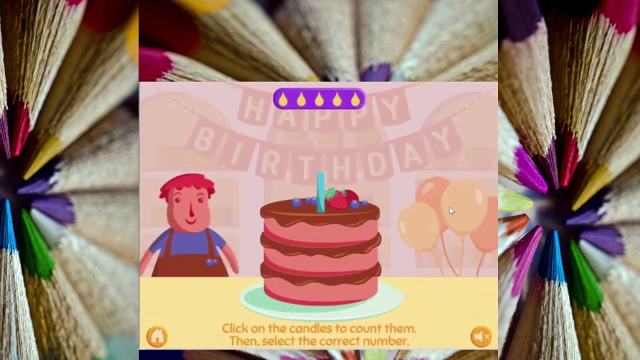 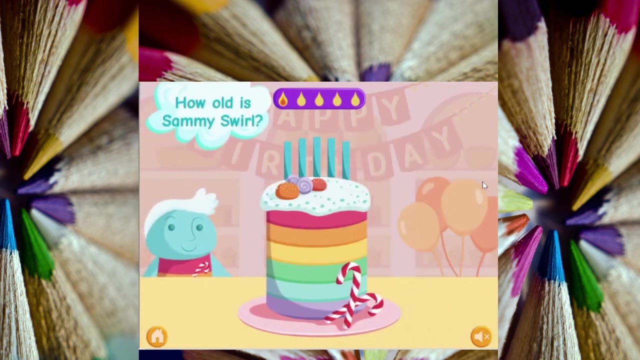 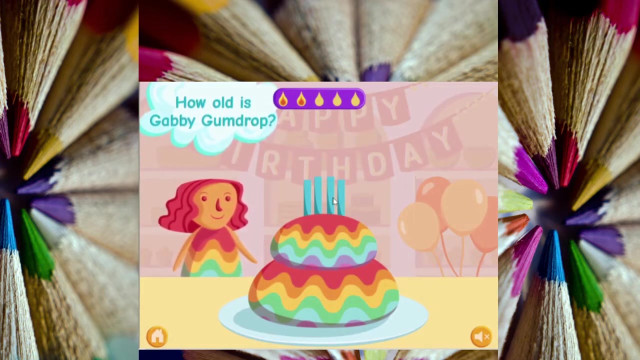 Click on the candles to count them, then select the correct number. How old is Dunkin' Donut? One. How old is Sammy Swirl? One, two, three, four, five. How old is Gabby Gumdrop? One, two, three, four. 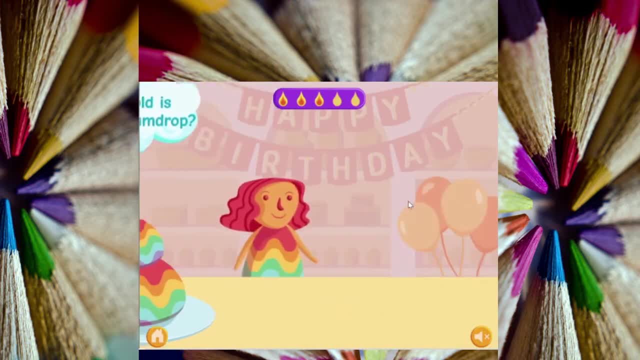 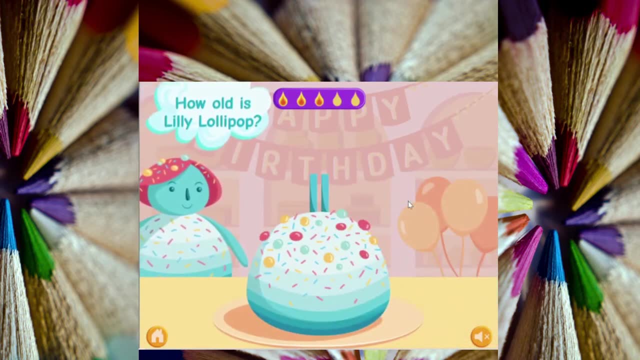 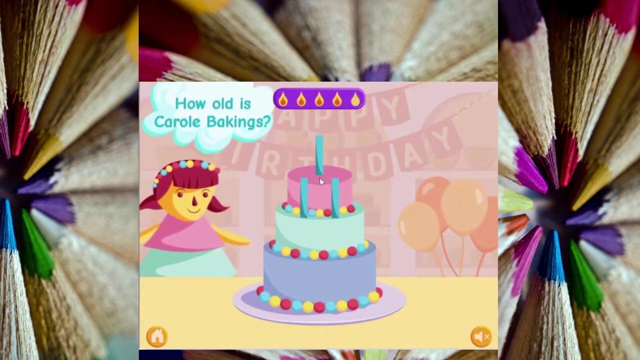 How old is Lily Lollipop? One, two, three, four, five. How old is Rosie condition? One, two, three, four, five. How old is Ellie? One, two, three, four, five. How old is celle? One, two, three, four, five. 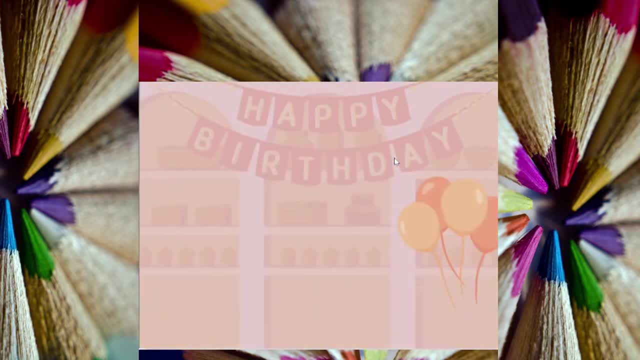 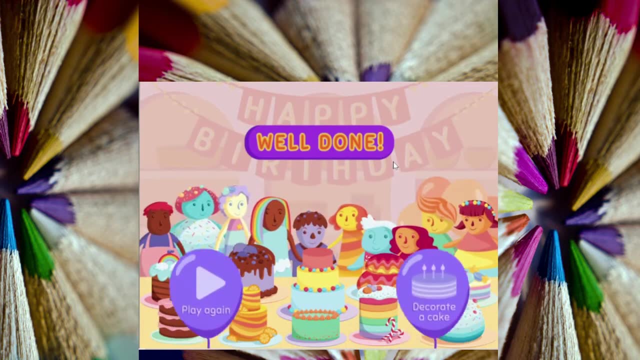 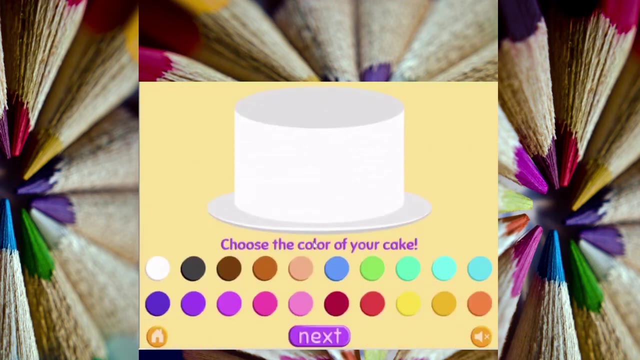 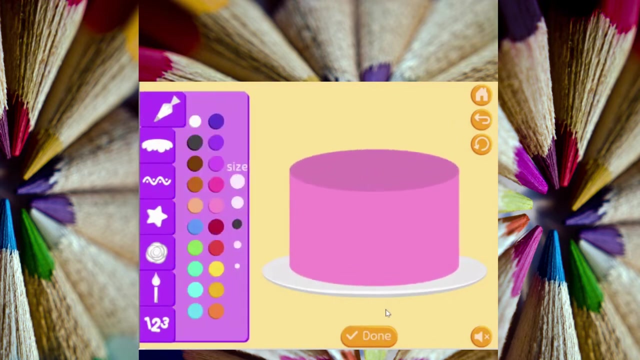 How old is Emily? One, two, three, four, five? Do you want to play again or decorate your own cake? Do you want to play again or decorate your own cake? Do you want to play again or decorate your own cake?